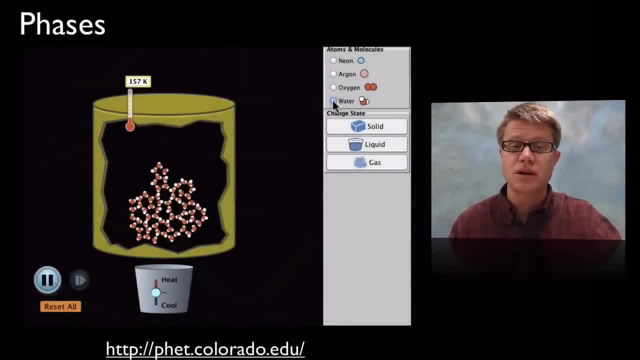 Or if you just turn that around a cooling curve, And it's going to show us this transition between the two. And so if we're looking at phases of matter, it's first best to come up with some kind of a representation of what they look like. And so we're going to use 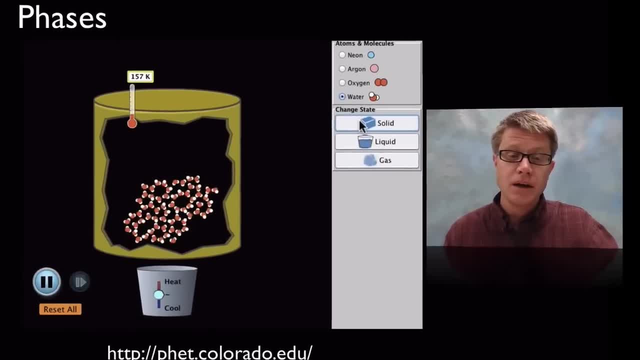 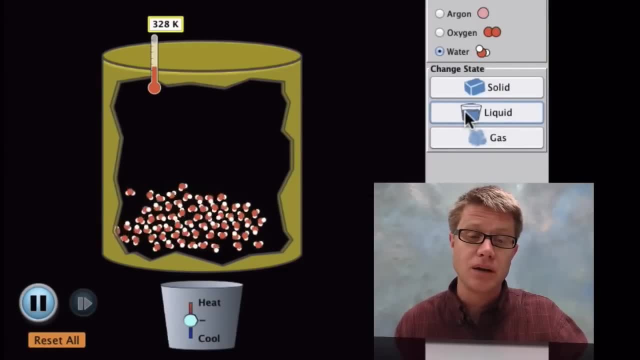 a simulation here from PHET at Colorado EDU, And so what we've got here is a bunch of water in a solid phase, And so you can see that they're locked in position And as we move it to liquid, now they can translate, They can move around each other. Now, this is not. 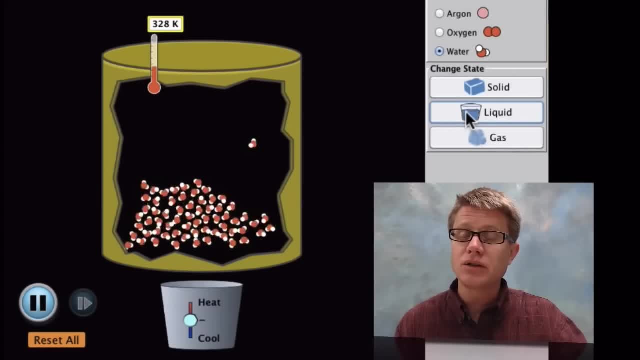 a great model of a liquid. It should kind of flow down to the bottom, But at least we're seeing what's going on at the bottom, At the particle phase, And then as we look at a gas, as we increase the energy again. 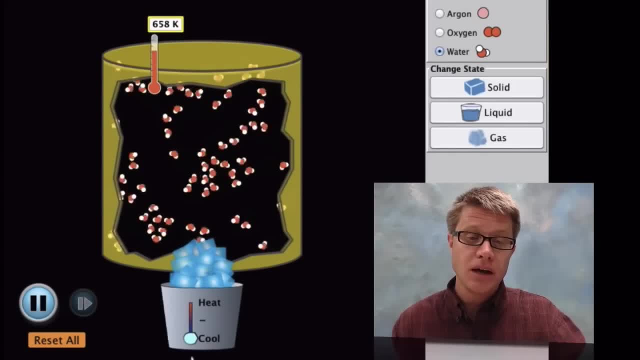 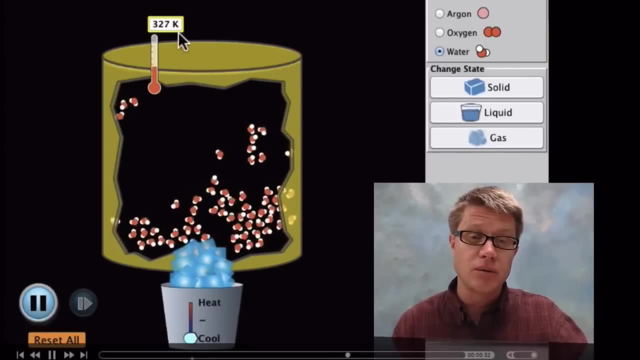 now. they're moving all over the place, And we'll talk about gases in the next video, And so what we're going to do is we're going to take some of that energy away. We're going to take some of that heat away And, as we cool it down, you can see here that we're measuring. 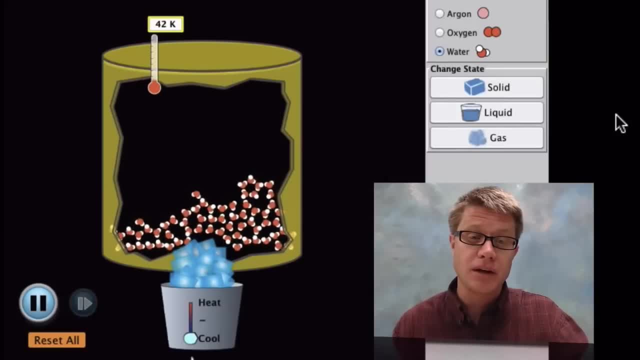 this in kelvin: As we cool it down, it turns into a liquid, And now it's into a solid. You can see, even at a solid phase, though, still we're seeing vibrations within there, But as we approach absolute zero, all molecular motion is vibrating, And that's what we're. 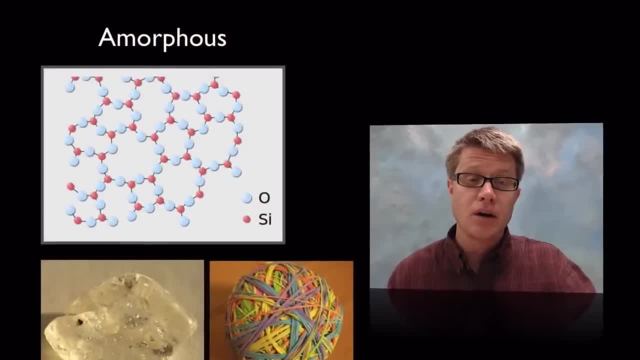 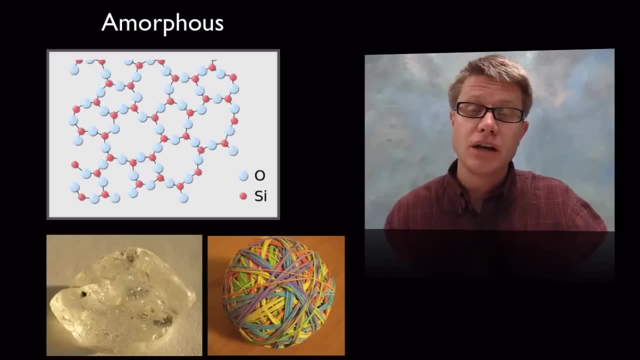 eventually going to come to a stop when we reach that point. Okay, So when we're looking at solids, solids are going to have a specific matrix. In other words, all of the atoms, molecules, are going to be put together in a specific shape. If 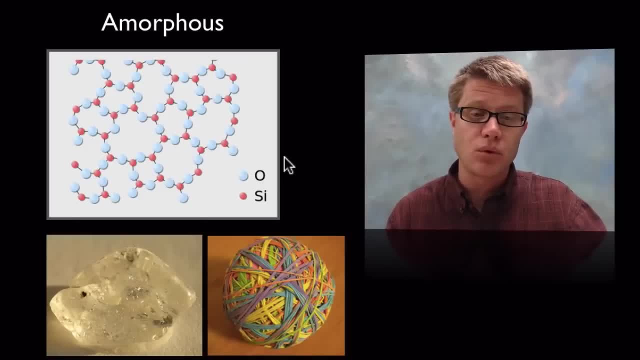 it's amorphous. there's not going to be a repeating pattern to this, And so this is amorphous right here. So you can see it's made of silicon and oxygen, But they're going to be put together in all different shapes And, as a result, we get what's called amorphous quartz, Or sometimes 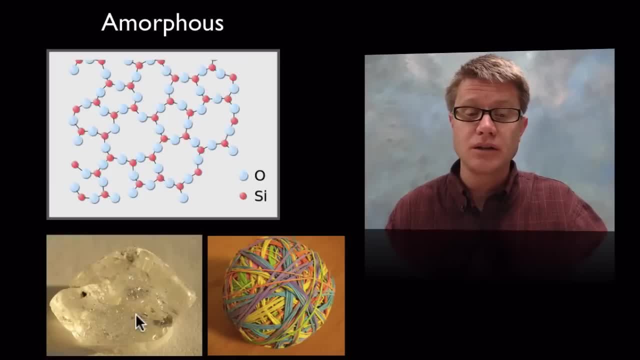 we call this glassy quartz, And so it's going to be really brittle, Really easy to break, And so it's going to be really brittle, Really easy to break, And so we're going to take this and we're going to take this, and we're going to take this, and we're going to take this. 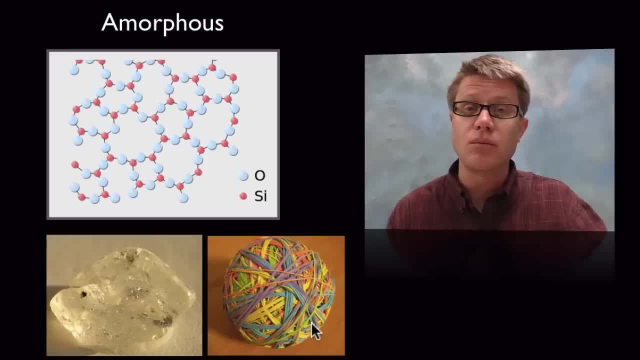 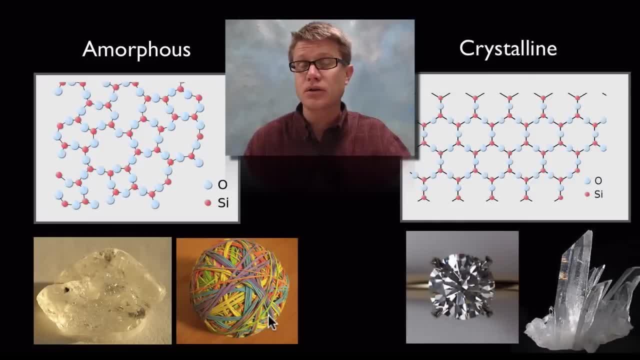 mean that it's not a solid. It's just not going to be as organized. And if we look at crystalline structure like that in this crystalline quartz it's going to be the same atoms you can see, But they're arranged in a repeating pattern And now we get these beautiful crystals. 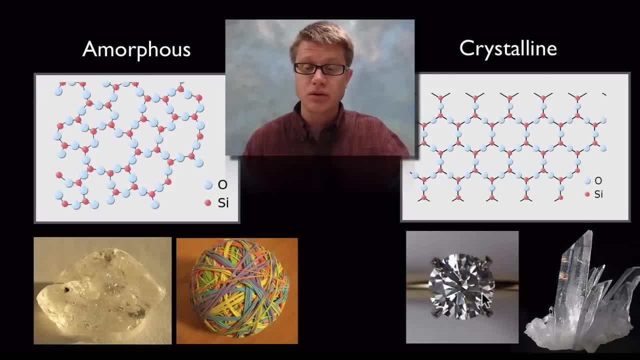 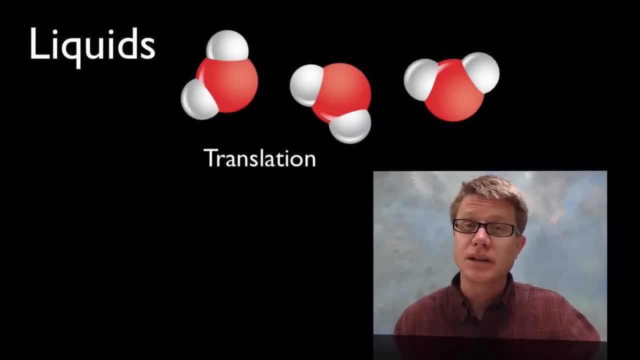 right here, It's going to be harder. So a diamond, for example, is going to be something that would be in a crystalline solid. As we move into liquids, what they can show is something called translation. So that means that let's say we have these two. These two are the. 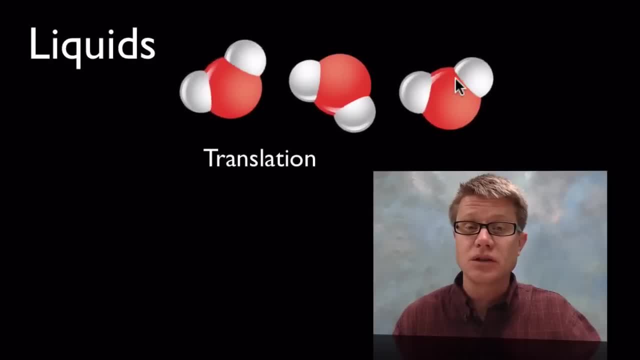 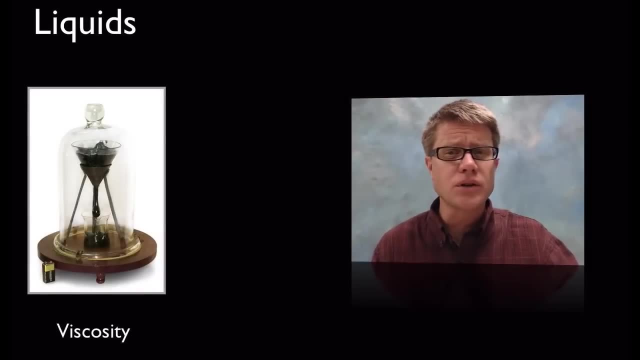 these water molecules right here. They're not locked in those positions. In other words, they can translate about each other And, as a result, liquids are going to take the shape of their container. Now, depending on the forces between those water molecules, we're going. 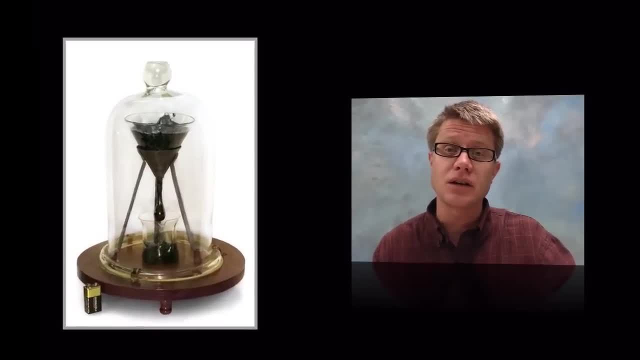 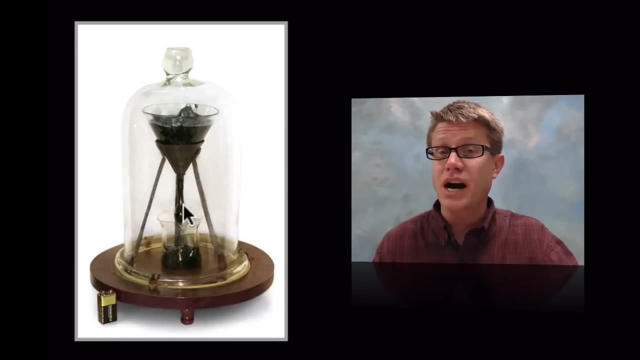 to have different properties. One of the first ones is going to be viscosity. Viscosity is how easily a liquid is able to flow, And so right here we've got a picture of pitch. Pitch is going to have really high viscosity. That means it really is going to flow at a real 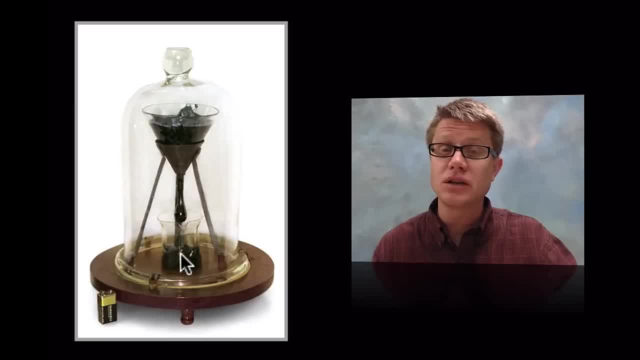 slow rate. It's still going to take the shape of the container you can see down here, And so something that would have, for example, a real low viscosity might be water. It's going to easily flow. Alcohol might be one that has a low viscosity. Another property is going. 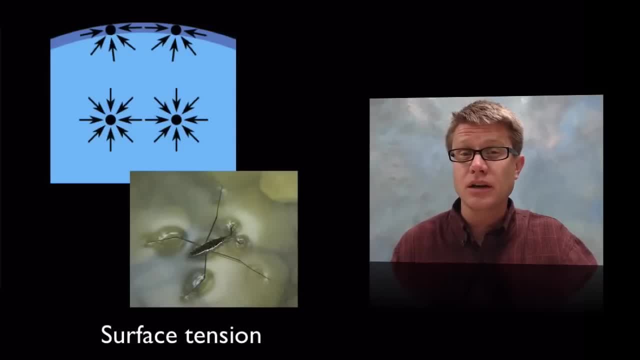 to be surface tension. Surface tension is going to be based on the intermolecular forces in a liquid, And so these different molecules are going to be attracted to one another, And they're also going to be attracted to one another at the surface, And so surface. 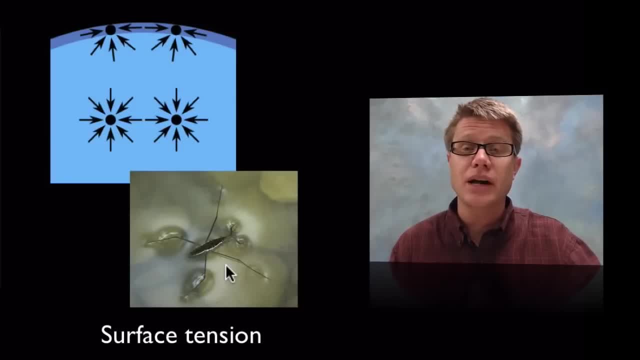 tension is going to be almost this layer of chemical attraction over the surface of a liquid, And that's what we're going to be talking about in a little bit. And then we're going to be talking about water, And so a water strider like this is able to float. 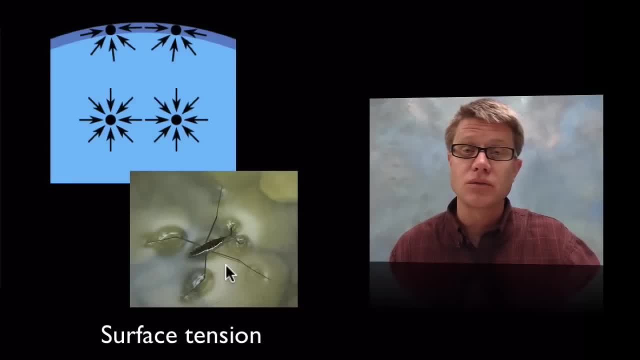 on top of that surface tension. If we were to break the surface tension, one way to do that would be to add something like soap. It's going to break those intermolecular forces And, trust me, that water strider is going to quickly sink to the bottom of the lake. 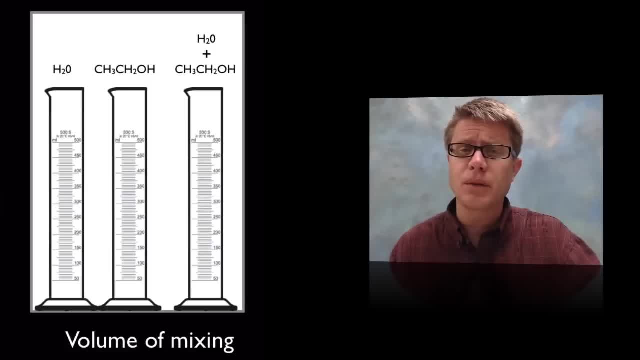 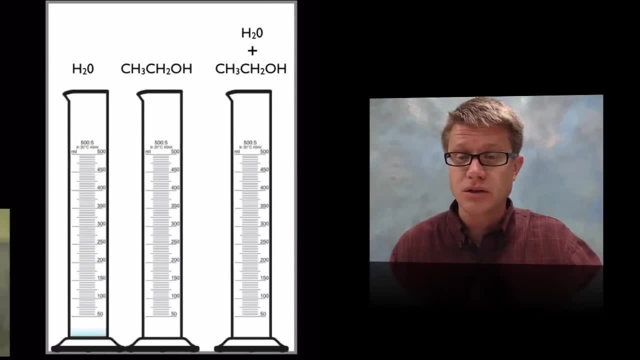 And then the last thing is called the volume of mixing, And this is it's best easily understood if we use a demonstration. This is one that I use in my class. Imagine I were to take some pure water, So we have distilled water, And I were to put it in a graduated cylinder. 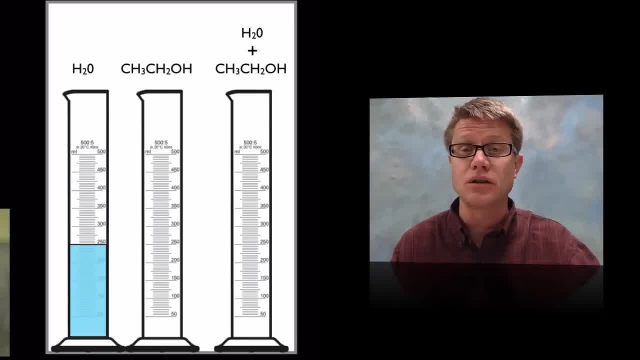 And I were to be real precise and measure out a graduated cylinder, And then I would be precise and measure out exactly 250 mL of water. I were then to take some ethyl alcohol- so ethanol- And I were to measure out exactly 250 mL of that as well. So let's say I'm very 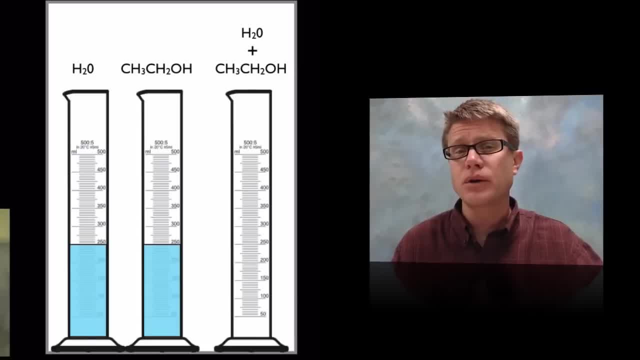 precise, I have 250 mL of each. What do you think is going to happen if we combine those two amounts together in another graduated cylinder? Well, when you do this, if you have a large enough amount, you're not going to get 500 mL, And so that's weird, It seems. 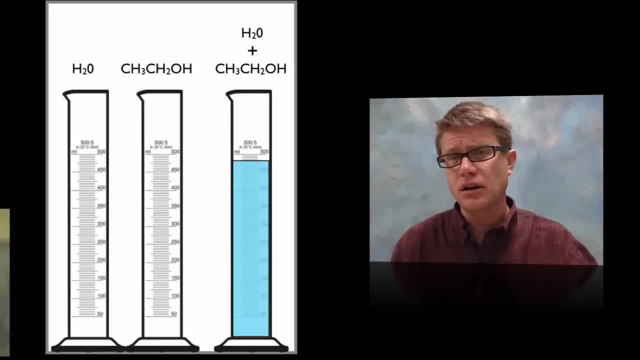